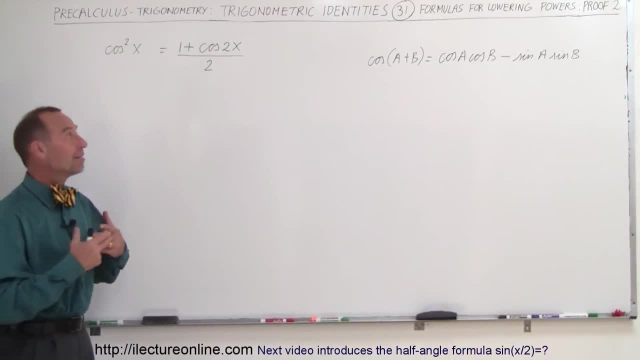 Welcome to Electro Online and here we're going to show you where the reduction formula came from for the cosine squared of x. Remember there's several identities or several formulas that allow us to change a sine or cosine or tangent function squared into a function to the first power. 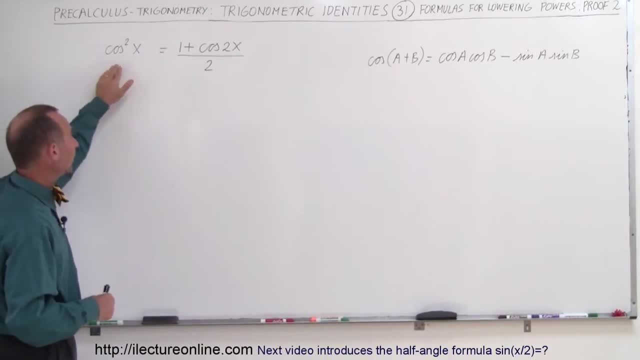 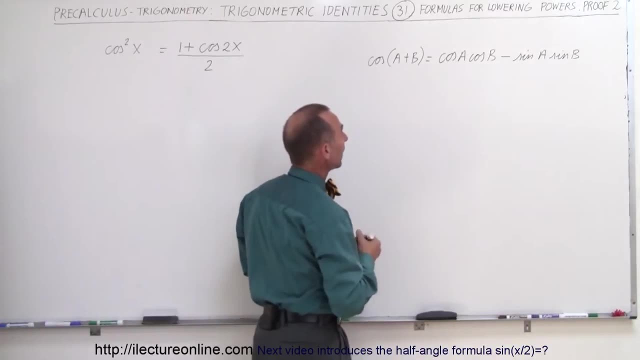 That's one of these reduction formulas. So where did this come from? How do we know that this is equal to that? Again, we'll start off with this identity right here, where the cosine of a plus b is equal to that, And so what we're going to do now is take the cosine of a plus a, So we're going to change every b to an a. 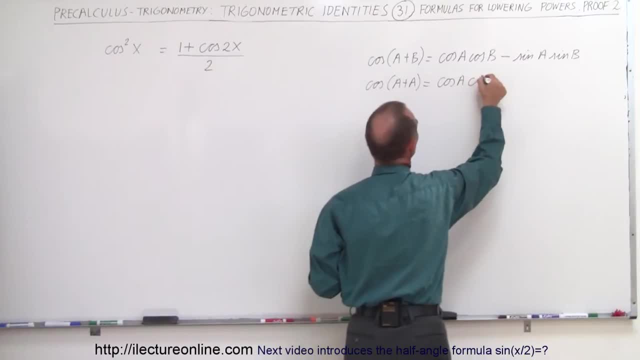 And when we do that we get the following: We get the cosine of a times the cosine of a minus. the sine of a times the sine of a- And of course that simplifies to the cosine of 2a- is equal to the cosine squared of a minus the sine squared of a. 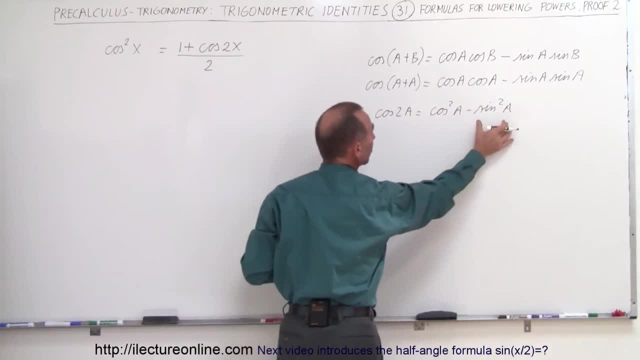 And of course then we want to solve that equation for the cosine. So we move this to the other side and we flip the equation around. so we have the cosine squared of a is equal to. So we get the positive sine squared of a plus the cosine of 2a. 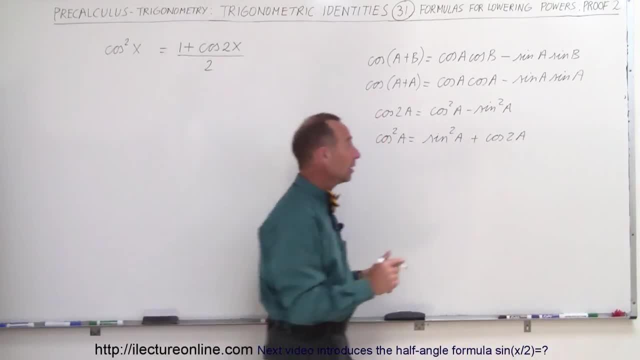 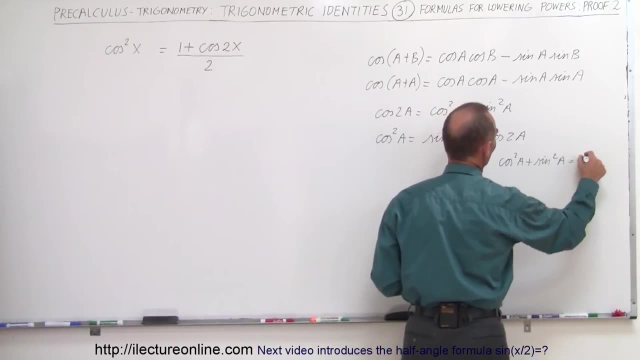 There, That's a better way to write it. So now again we go to the identity that everybody knows, that the cosine squared of a plus the sine squared of a is equal to 1.. This is probably the most fundamental identity in trigonometry, which allows us to write the sine squared of a as follows: 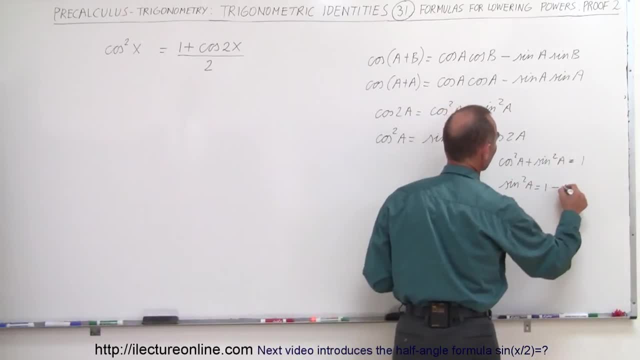 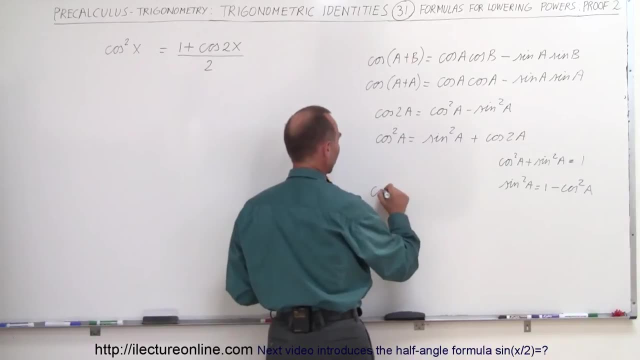 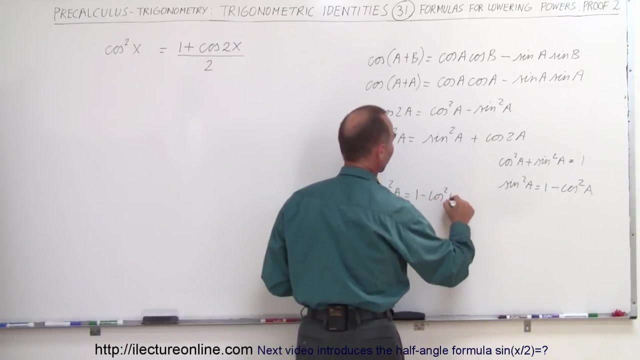 So the sine squared of a is equal to 1 minus the cosine squared of a. And then we substitute the sine squared of a by what it is equal to, right here. So now we can write that the cosine squared of a is equal to. instead of this, we write that 1 minus the cosine squared of a, plus the cosine of 2a. 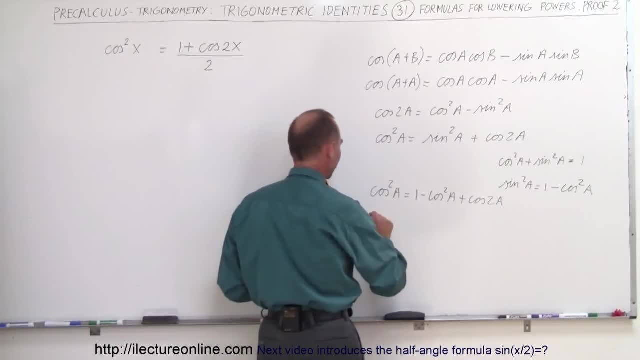 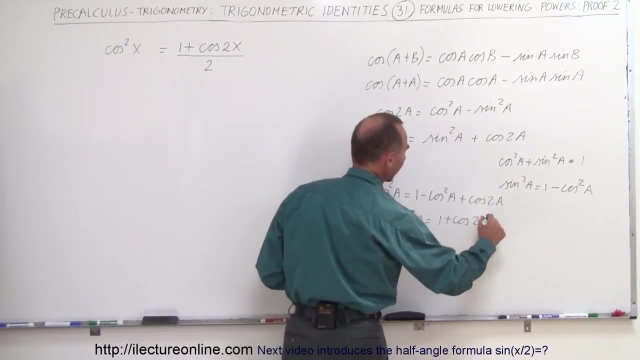 Then again we move the cosine squared of a to the left side, So now we have cosine squared of a plus the cosine squared of a is equal to 1 plus the cosine of 2a. now you can start seeing that this is beginning to look a lot like what we have over. 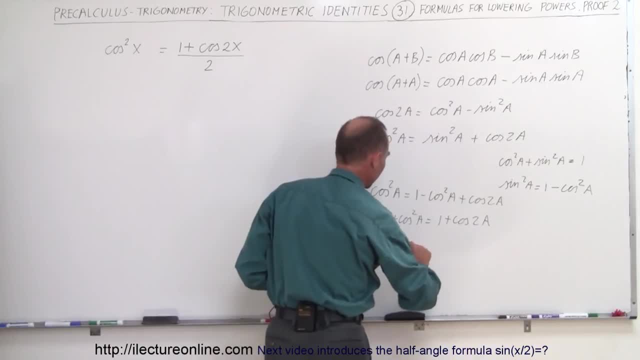 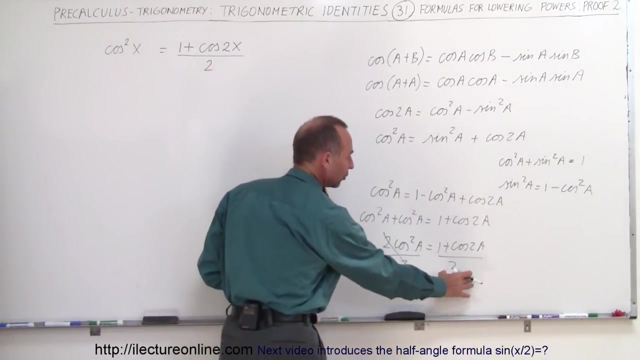 here. so now we have two times: the cosine square of a is equal to one plus the cosine of 2a. and then if we divide both sides by two, so divide the left side and the right side by two, this cancels out. and so now we have the cosine square of a is equal to one plus the cosine of 2a divided by two. 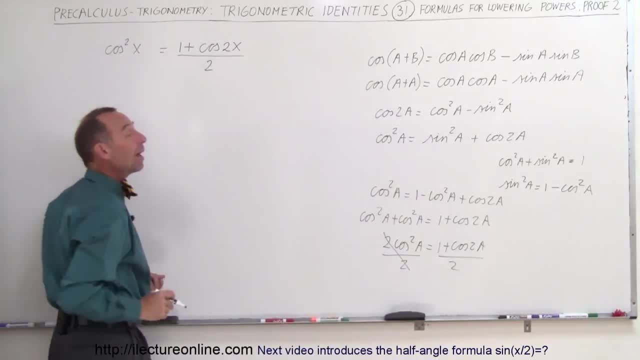 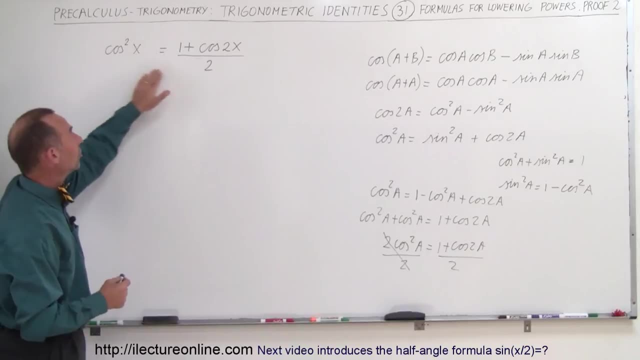 which is exactly the same what we have over here, except we use x instead of a. but again, that's where that, that formula comes from, that identity comes from. so here we have proof that this is equal to that, and now we can use it. 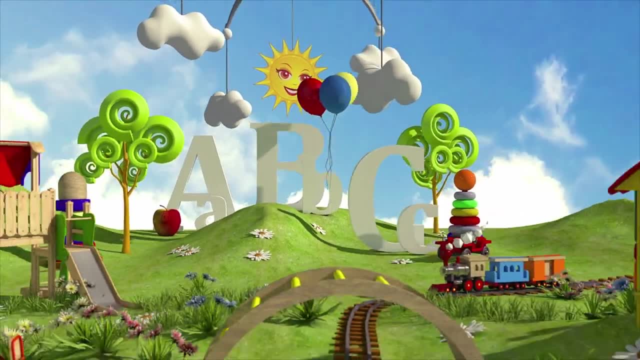 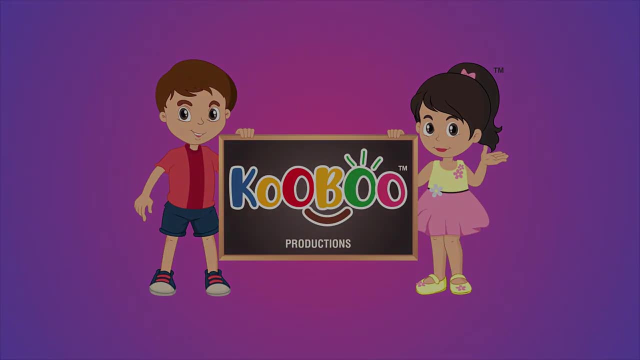 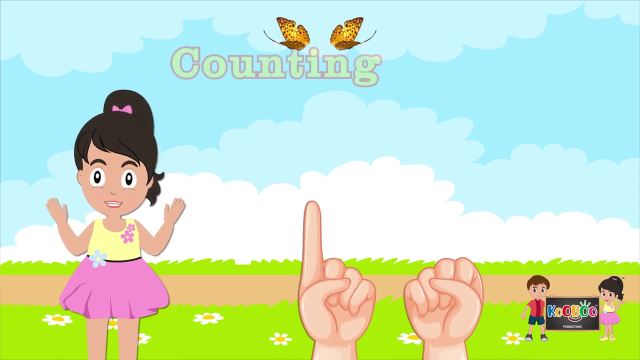 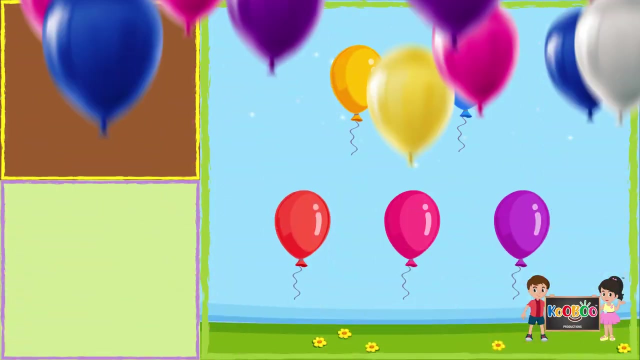 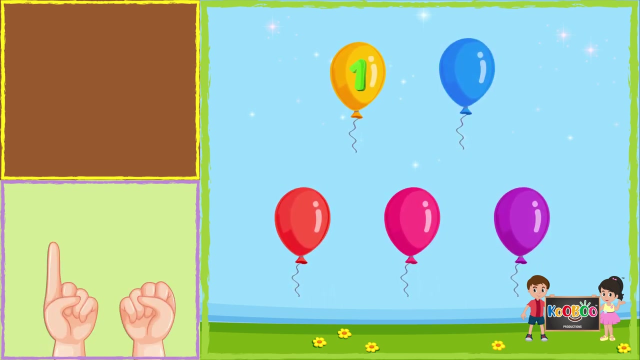 Hi kids, I am Boo. Today, let us learn how to count numbers with the help of objects. In the first image we see how many balloons Let's count: 1,, 2,, 3,, 4 and 5.. So we found. 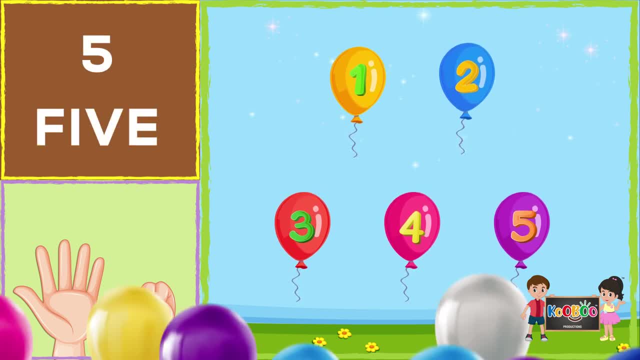 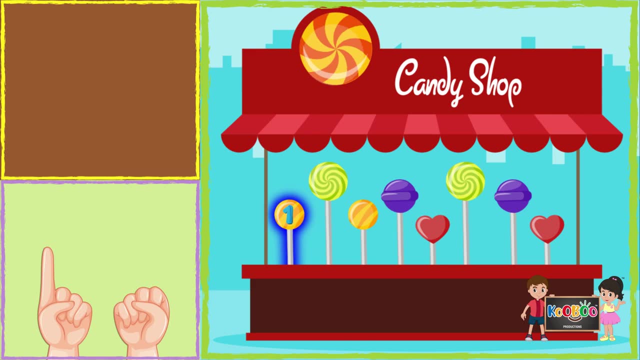 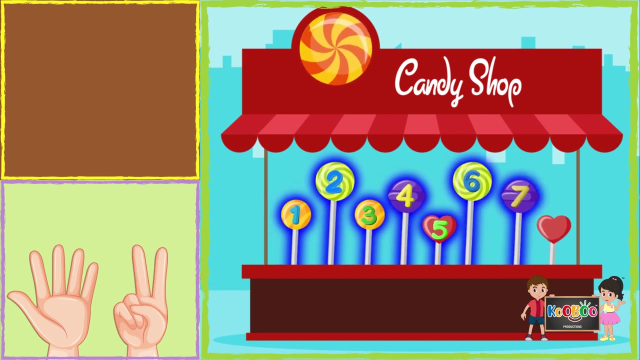 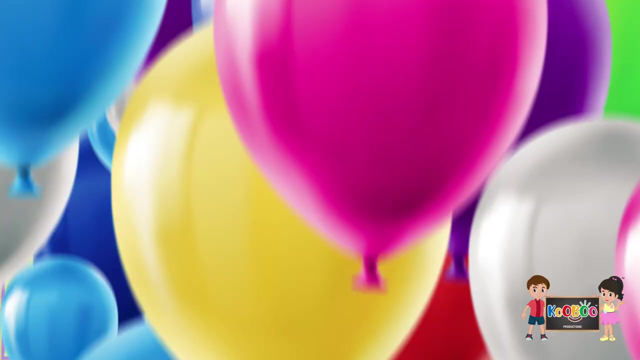 5 balloons. Next, in the second image, we see how many chocolates: 1,, 2,, 3,, 4 and 5.. 4,, 5,, 6,, 7,, 8.. So we found 8 chocolates. In the third image we see how many flowers. 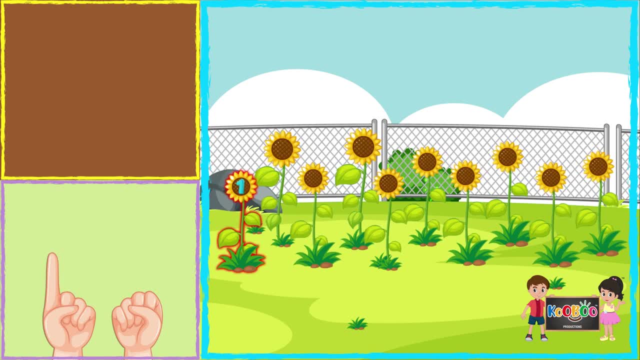 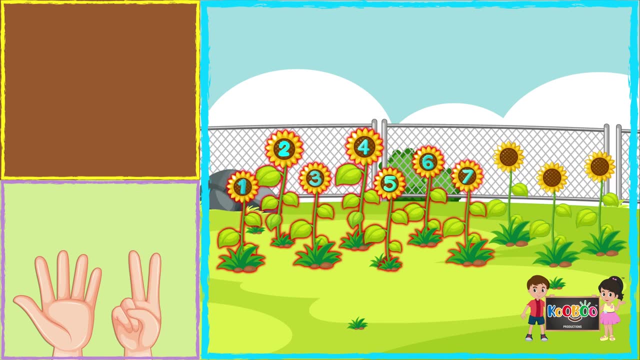 Let's count 1,, 2,, 3,, 4,, 5,, 6,, 7,, 8,, 9,, 10,, 11,, 12,, 13,, 14,, 15,, 16,, 17,, 18,, 19,, 20,, 21,. 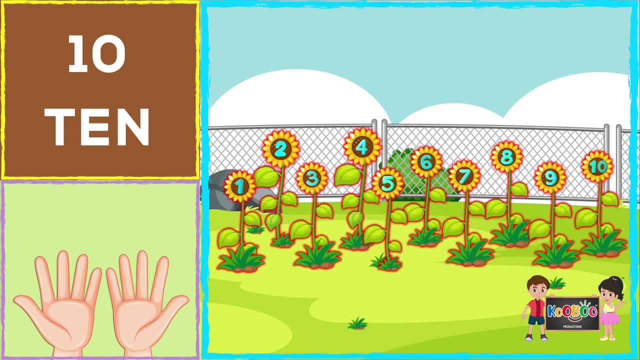 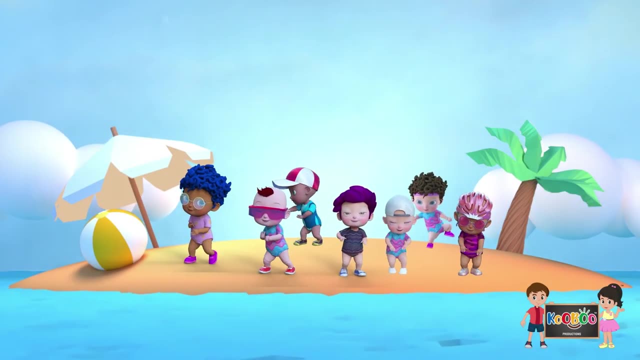 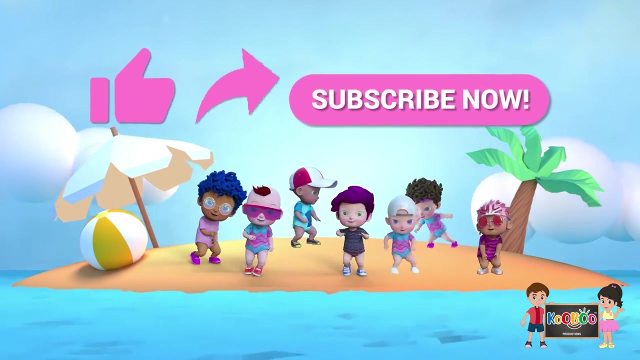 22,, 23,, 24,, 25,, 26,, 27,, 28,, 29,, 30. So we found 10 flowers. See, kids, it is very easy to count with the help of objects. Do practice counting at home and have fun.